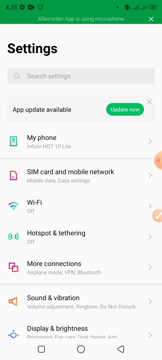 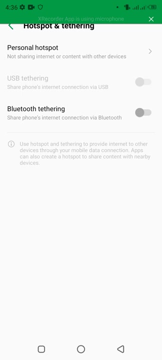 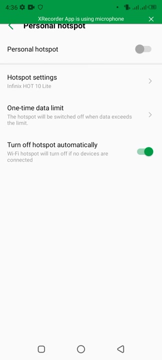 versions that you can take advantage of. okay, so let's begin. so to begin with, you on your hotspot, turn it on. so here is the hotspot. on other phones might be different name, but here is personal hotspot. so you click on it, then it will take you to the setup page. so before you use it, you turn. 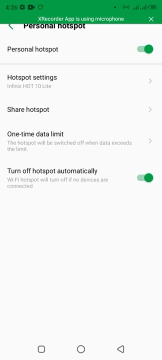 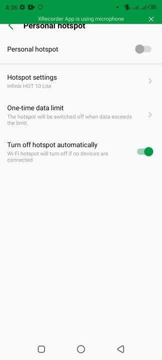 it on by ticking this. so it's now on. but before that, I want to show you the trick that can make you to limit your data consumption over this hotspot. so so I'm going to show you how to do. I'm going to turn it off, then, before then you can set it up. the creator, you want to put it, the- 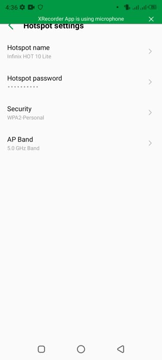 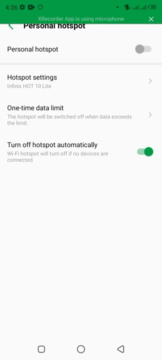 password you want, you can put it here. and the band, the network bandwidth, you want it. that to all. two point four or five, so mine is on five. okay, now the cool feature I want to show you is how you can limit the data that the person that is turned on your hotspot for we use. 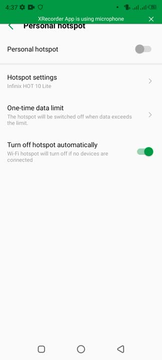 so here is it. so you can see there is something written here: one time data limit. so that is where the trick comes from, so I will click on it. once you click on it, you can see a toggle button here to turn it on. but before turning it on, here is the trick here. so the trick here is this data limit as 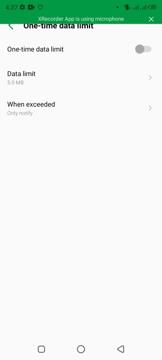 you can see, there's a data limit on it which is five. so what here means? what this means is that you can turn off the hotspot for the person and you put the data limit at five. so once the person exceeds this data limit, that means if you turn this toggle on the data, the hotspots would off. 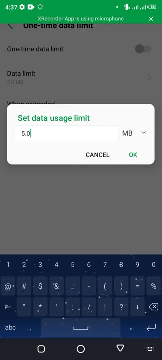 automatically, without you touching it. so if you put it on 30 megabytes for the person, or even 100 once it gets to that point, once it gets to the 100, when the person exceeds this- before you can't exceed this, but before you exceed this- it will turn off automatically and you can see the data.